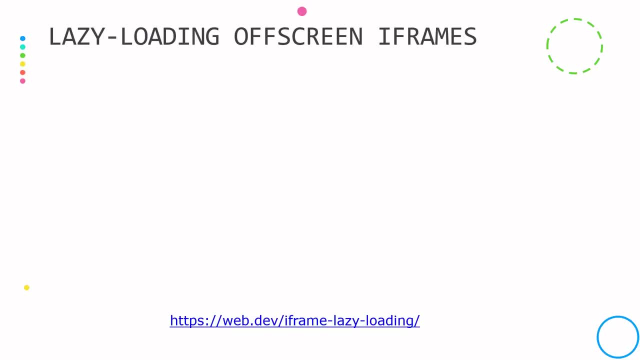 In my previous image optimization video I had discussed about lazy loading images and how it is helpful in page speed and website performance. Similar to that, lazy loading iframes defers the iframe being loaded until the user scrolls near them. That is, it display the iframe element only when the user scrolls down and reach that particular viewport. 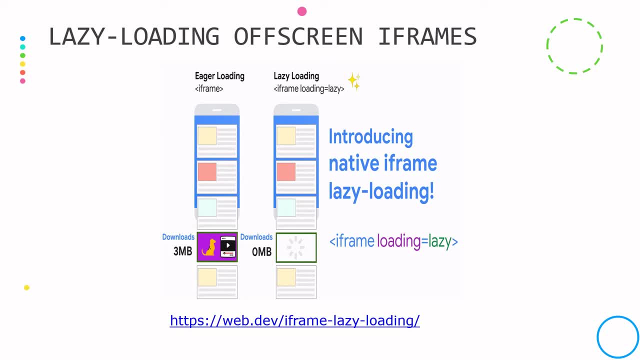 For example, iframe iframe. in this image you could see eager loading iframe and lazy loading iframes. In eager loading iframe you could see the off-screen iframe elements which is under the mainfold or loader, and it took 3 MB to download the element. It is not yet visible to the user because they not yet scroll down, but the iframe element is available, Whereas in lazy loading. 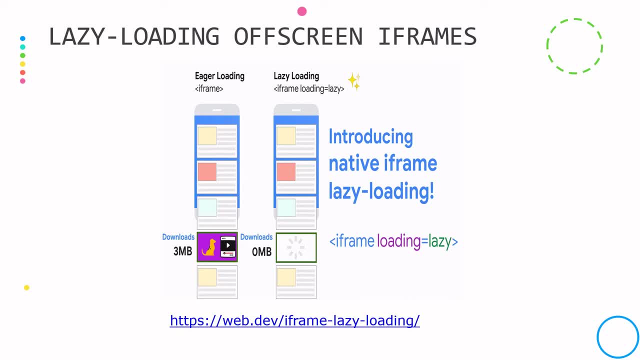 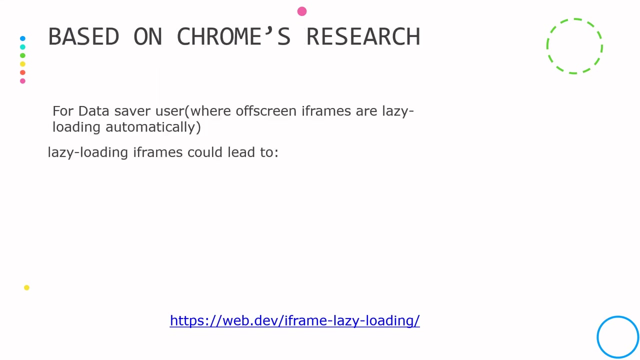 iframe. you could see the off-screen iframes are lazy loading. it is not yet loaded and it is available only when the user scrolls down and reach the viewport. by lazy loading off-screen iframes, it helps to saves data, improves the website performance and it reduces the memory usage. based on Chrome's research. 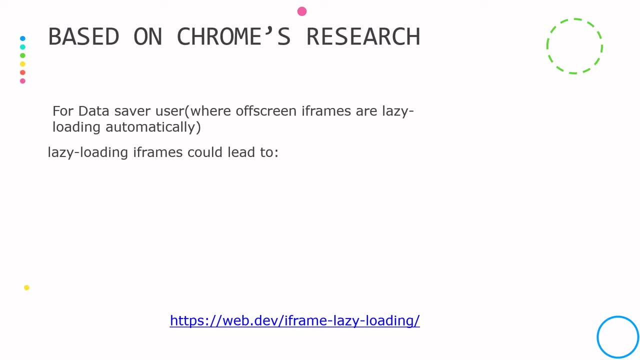 in data server mode where off-screen iframes or lazy loading automatically. lazy loading iframes could lead to two to three percentage median data savings. one to two percentage first contentful paint reduction at the median and two percentage first input delay improvements at the 95th percentile. I 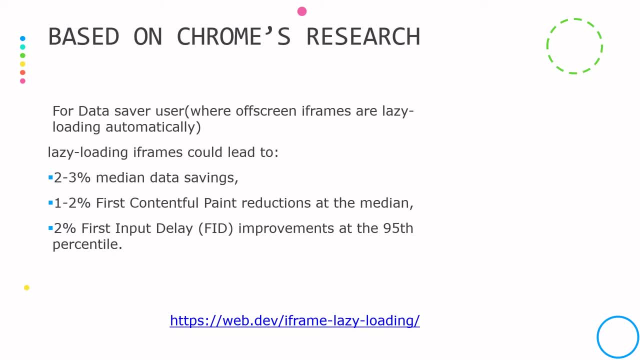 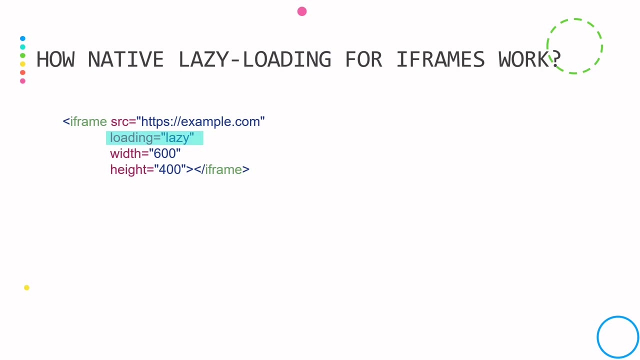 hope, using iframe lazy loading, we could improve two metrics- FCP and FID. and I hope, using iframe lazy loading, we could improve two metrics, FCP and FID, thereby improving Google PageSpeed insight score. okay, how native lazy loading for iframes work. the loading attributes allows the browser to defer. 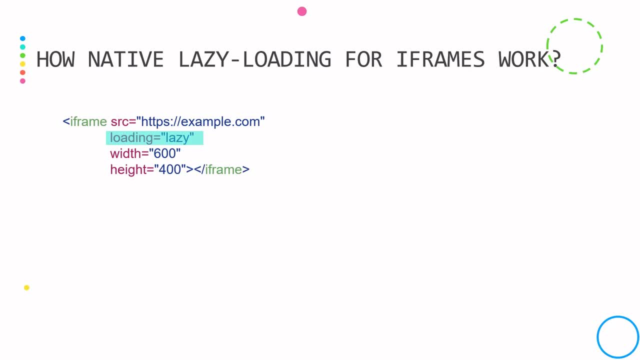 loading off-screen iframes and images until the user scrolls near them. the loading attribute supports three value: loading, lazy and loading either. loading auto: it lazy- load the off-screen iframes in loading eager. it loads right away the. of it lazy- load the off-screen iframes in loading eager. it loads right away the.